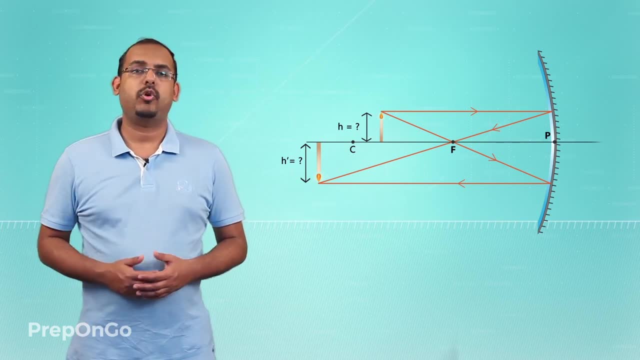 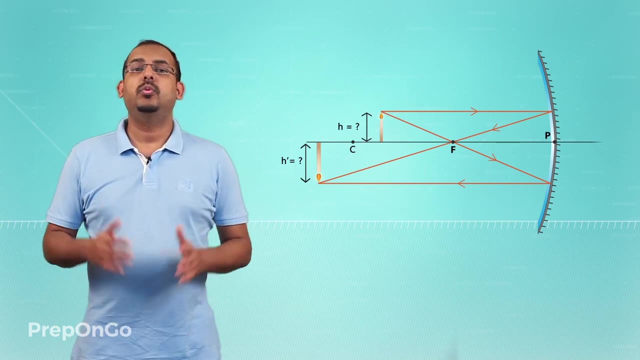 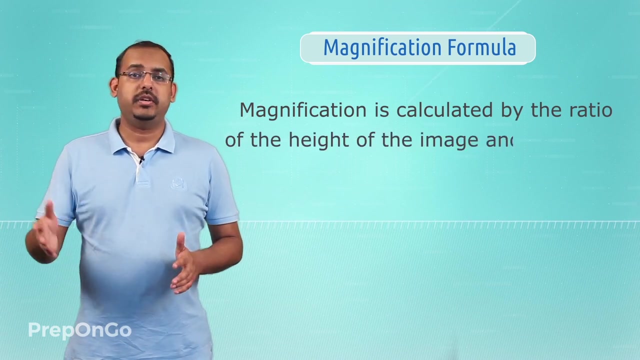 of an object with the help of spherical mirrors becomes very important too. The magnification of an object with the help of a spherical mirror is measured with the help of an expression which is known as the magnification formula. So the magnification formula is basically the ratio of the height of the image to the height of the original. 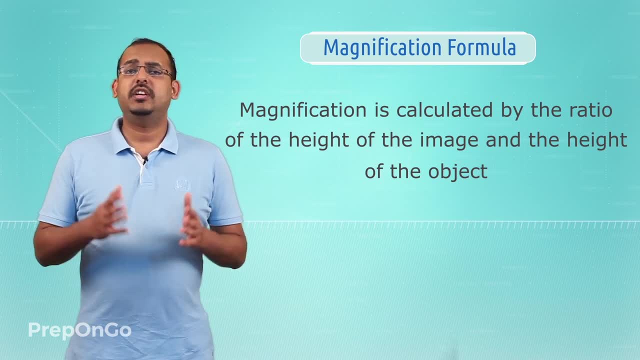 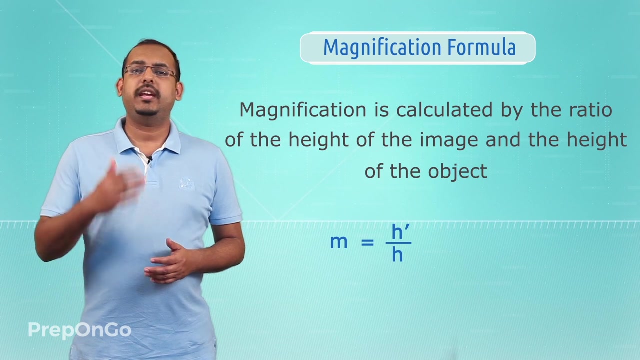 object. In simpler words, magnification is just the relative size of the image with respect to that of the object. In mathematical terms, the magnification is represented with the small letter M and is given by the expression. M is equals to h dash upon h, where h dash is the height of the. 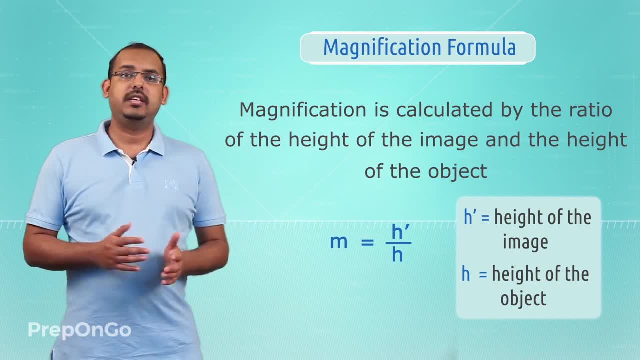 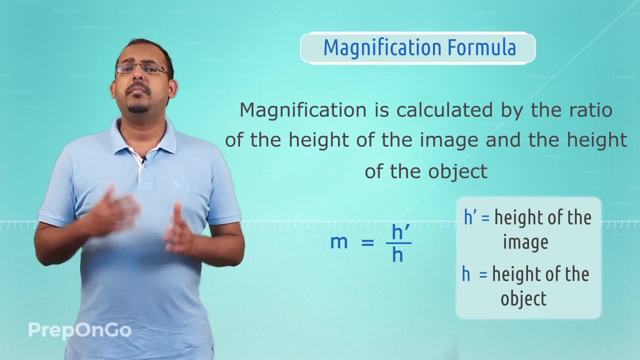 image that is formed by the spherical mirror, and h is the height of the original object. So magnification is the relative size of the image with respect to that of the object- original object, both taken with the appropriate signs according to the sign convention, The magnification of an image with respect to the object is also given. 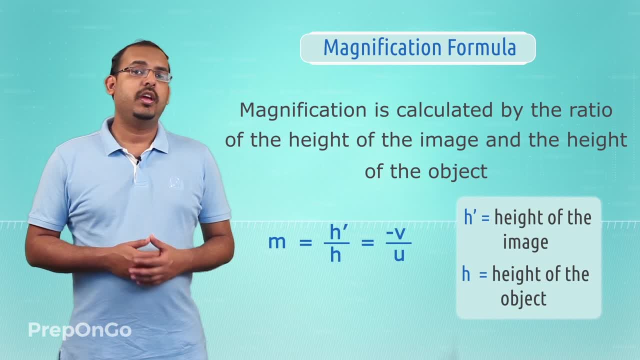 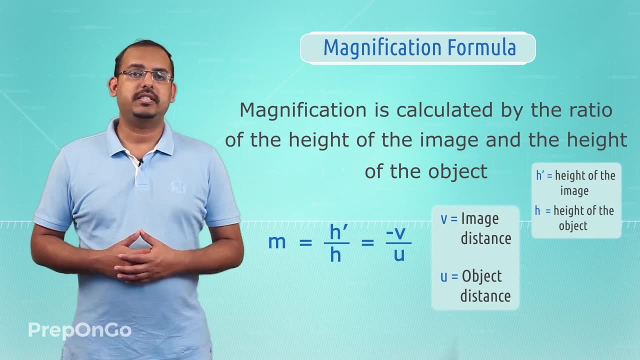 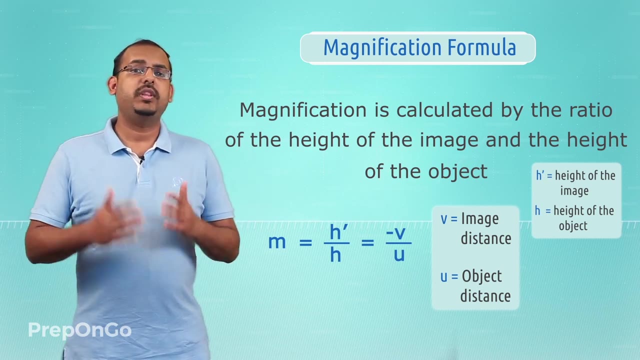 by the expression, m is equals to minus v upon u, where v is the image distance, with the appropriate sign, and u is the object distance, again with the appropriate signs. So, using any of these two expressions, we can calculate any of these five given unknown values with the help of the known values that we have. 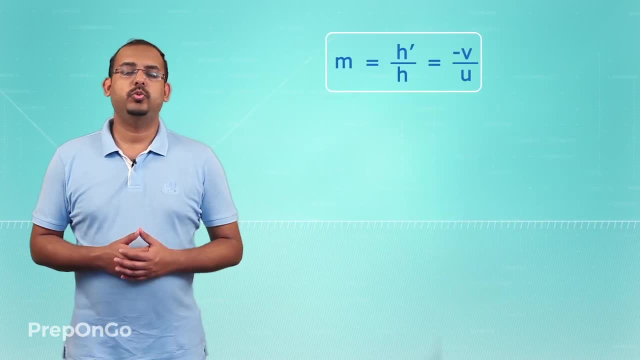 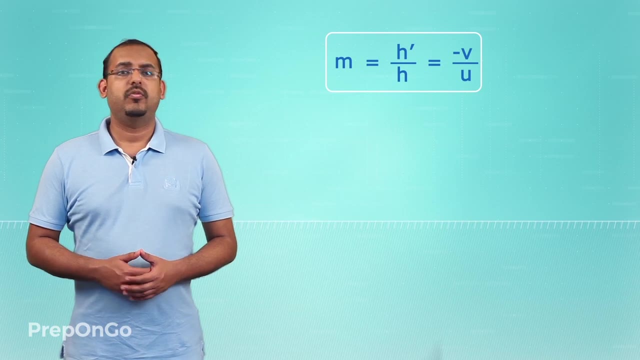 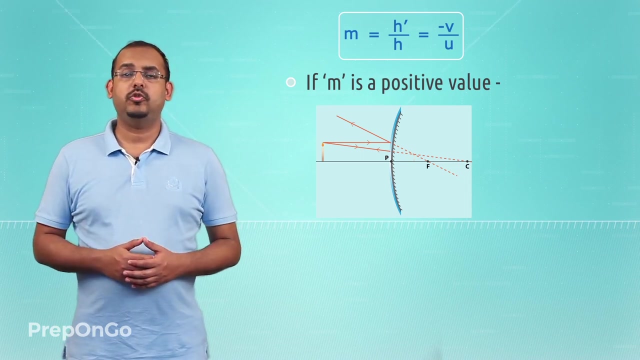 There's a lot more information that can be deduced out of the magnification formula. We can infer the nature of the image with the help of the magnification. well, if the magnification turns out to be a positive value, we can see that the image distance should also be a positive value, because we know that. 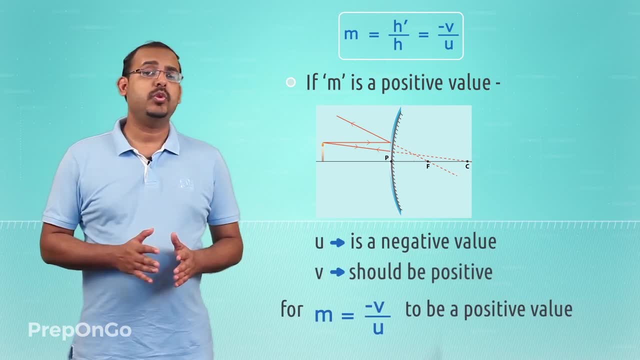 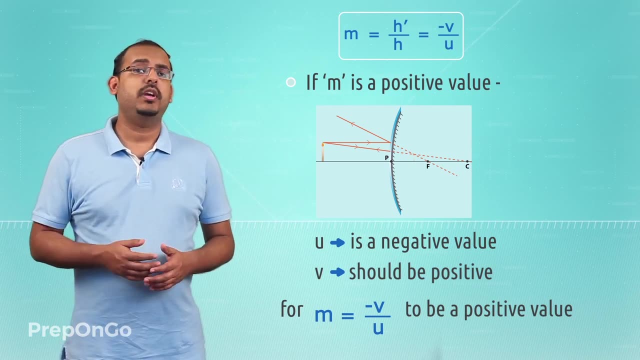 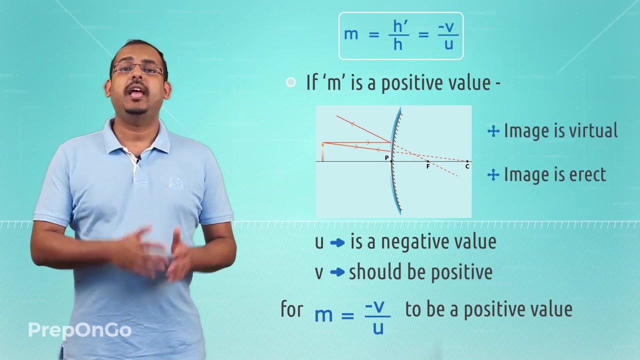 the object distance will always be a negative value, since the object is always placed on the left of the mirror. For the image distance to be a positive value, the image should be formed on the right side of the mirror. This implies that the image formed should actually be a virtual and erecting orientation. 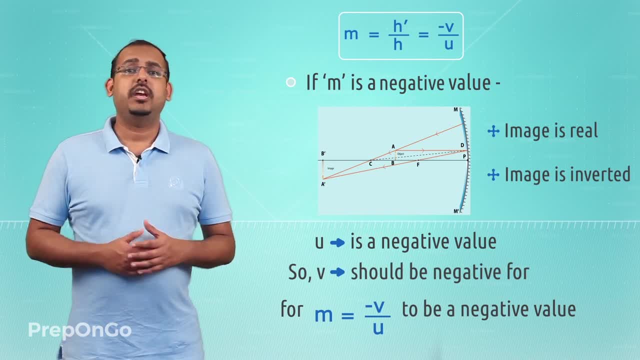 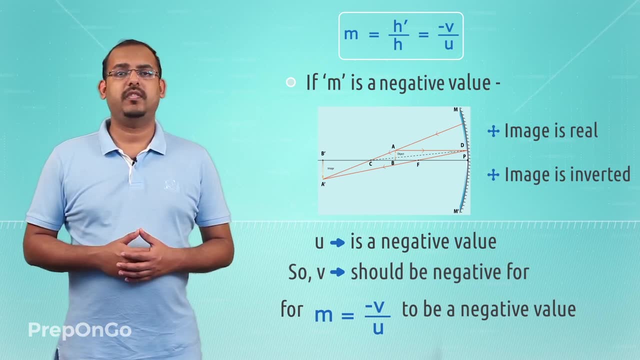 image. Now, similarly, if the image, if the magnification value turns out to be negative, then we can say that the image distance also has to be a negative value, which implies that the image should be formed on the left hand side of the mirror. 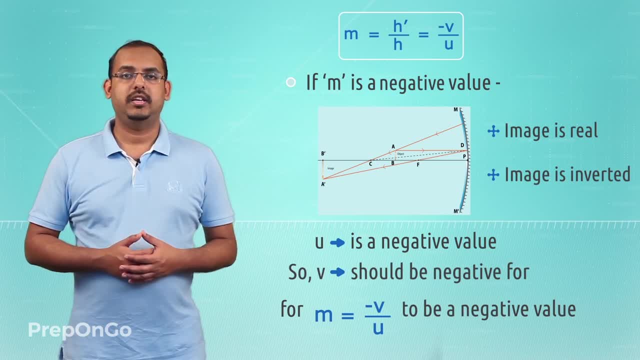 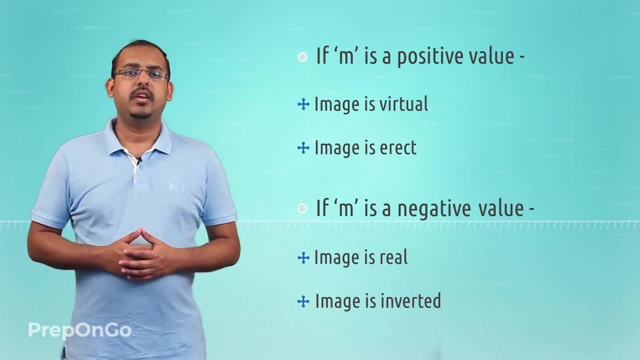 This means that the image form should be real and inverted in nature. So these are the basic concepts that are related to magnification of a biospherical mirror. Now we'll try to apply these- the magnification formula and these concepts, with the help of.